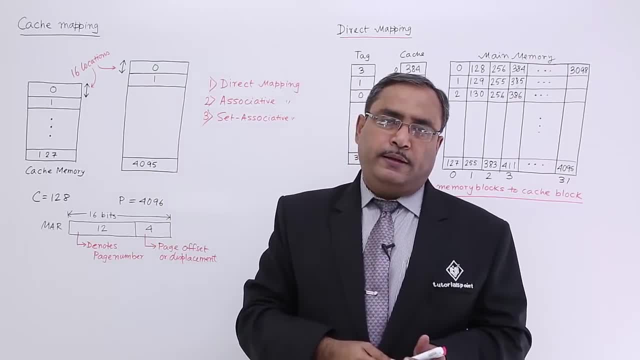 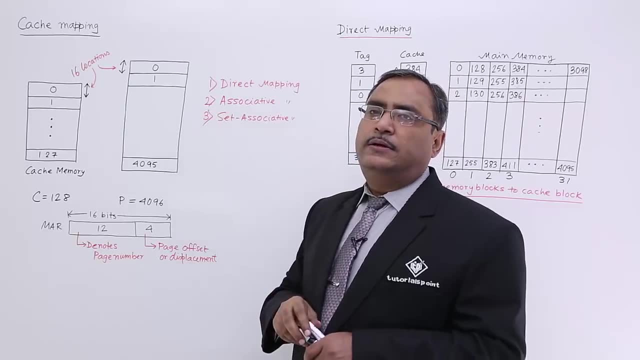 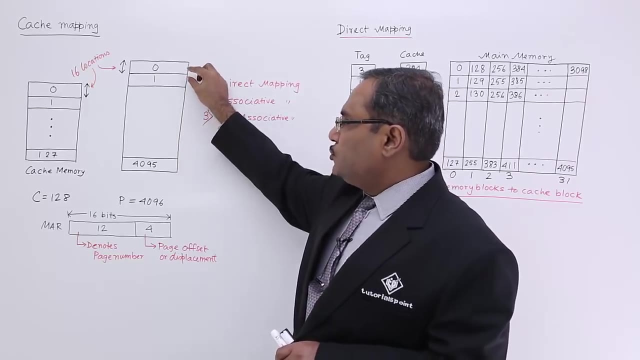 4096 number of pages. What is the page? The main memory, full main memory, will be divided into equi-sized fragments. Equi-sized, that means all these fragments are having the equi-size, same size. So if we go on dividing this main memory, then I shall get 4096. number of pages. 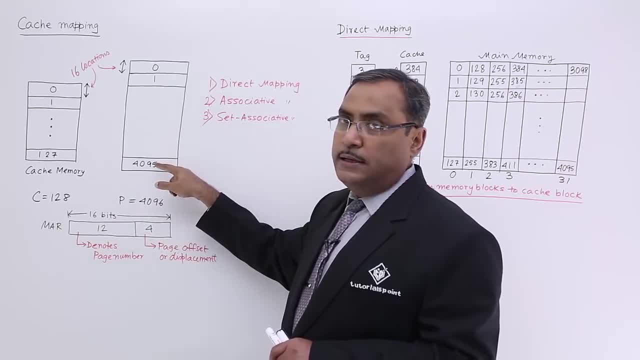 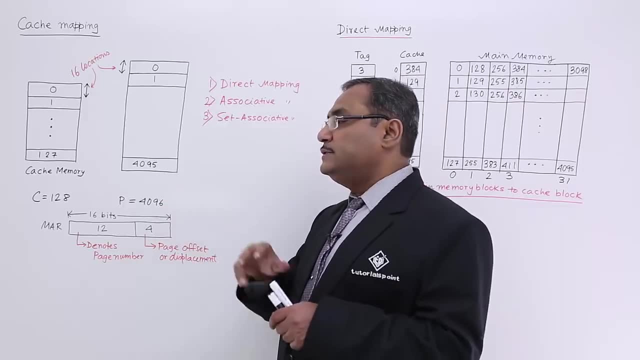 of, I shall get four zero nine six. number of pages, as I'm starting from zero, so that last page number has become four zero nine five, but if you go for the count, it is four zero nine six number of pages are there, so each and every page. 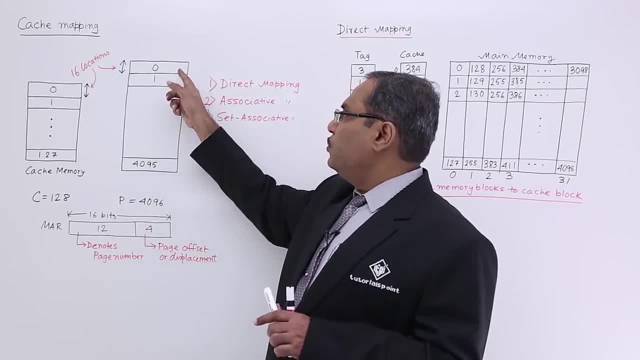 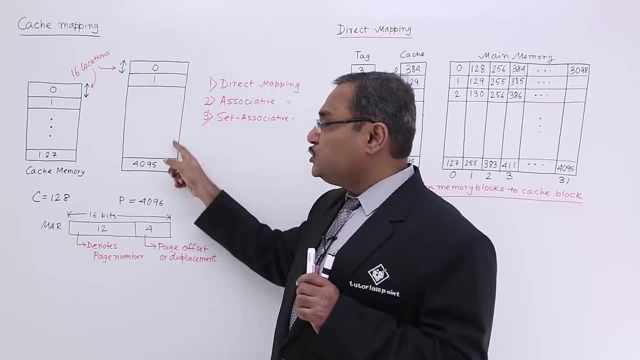 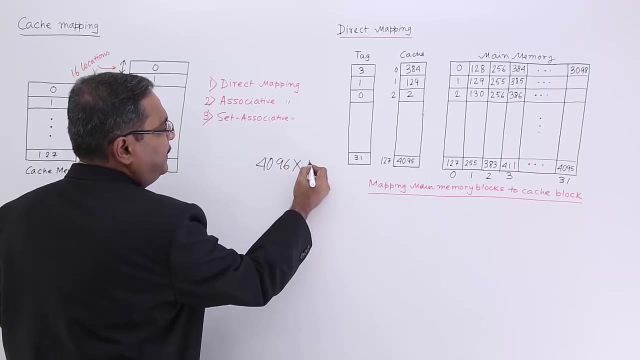 has got certain number of locations. so here this location number. I have considered that: 16 locations per page. okay, so that means how much memory we are having. how much memory we are having, we're having four zero, nine, six number of pages. each page is having 16 locations. so what is this? this is 2 to 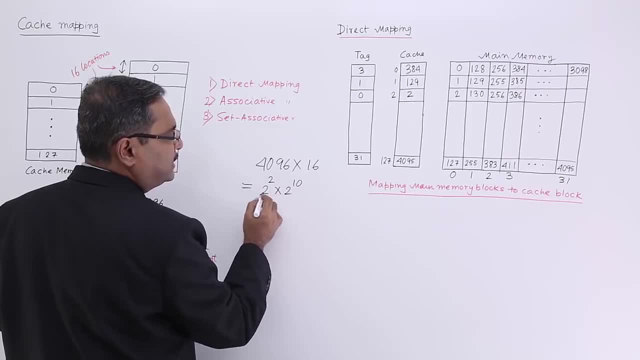 the power of 2 means 4, and 2 to the power of 10 means 1, 0, 2, 6. if you go on multiplying you are getting 4 0, 9, 6 into 2 to the power of 4 for 16. so we are: 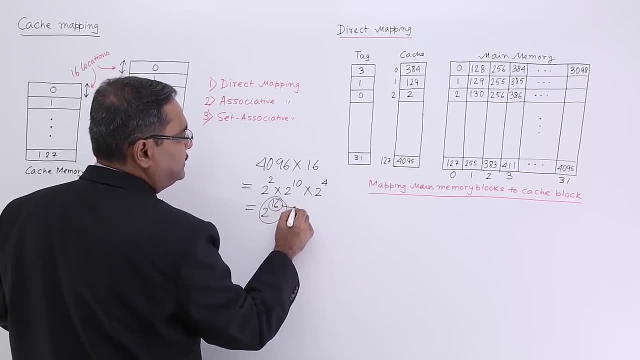 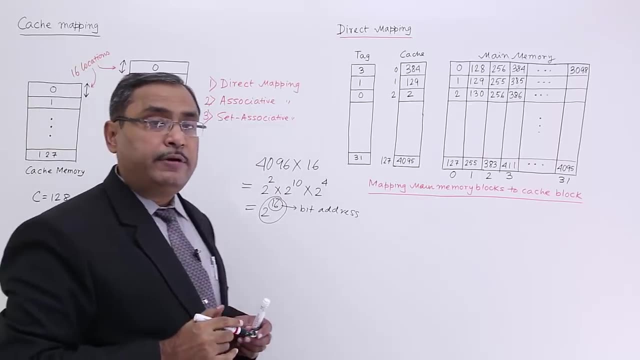 getting 2 to the power of 16, so actually we are having this 16-bit address. so this memory is having 16 locations. so we are getting 16 locations. so actually we are having 16-bit address. so now, if you consider this one, we are having 16-bit. 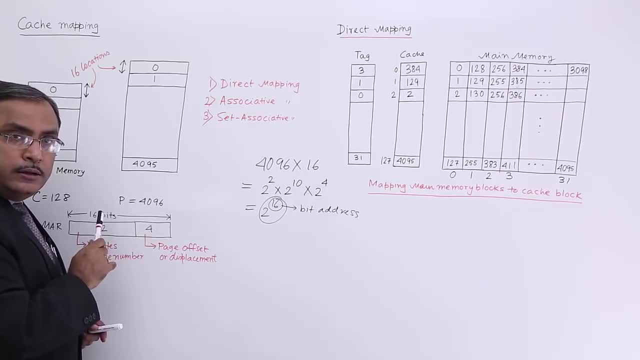 address. out of them, 12 bits will be denoting the page number and 12 bits can have combination to the power of 12. that is 4, 0, 9, 6. that is page number 0 to 4, 0, 9, 5, and here we are having 4 bit offset and it will be denoting the page offset. 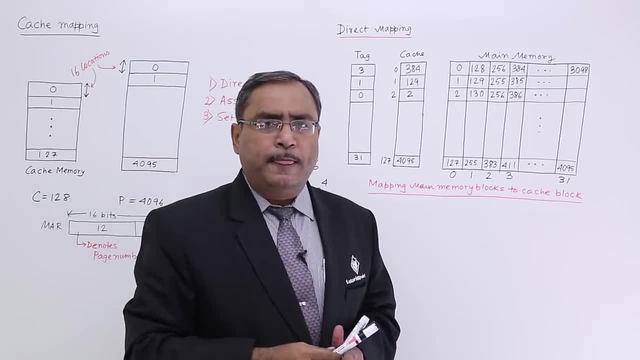 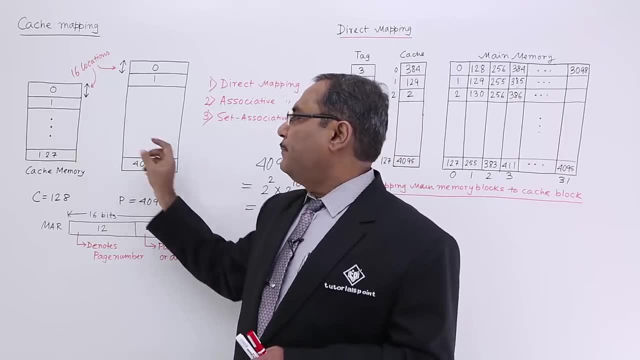 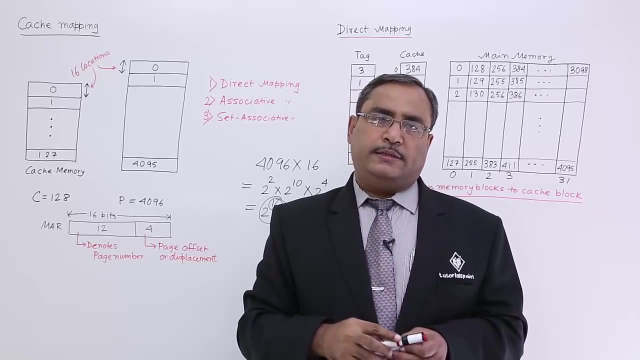 so that is a 16 locations per page we have taken. you might be asking me: why this? why not the single byte or single locations data is getting that white pagewise because you know that each and every program has got locality off reference. what is locality of reference? locality of reference is that the 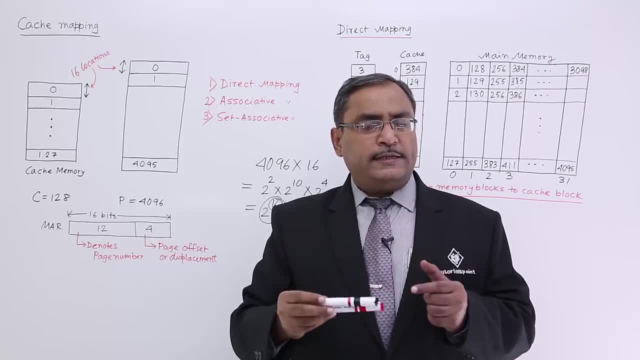 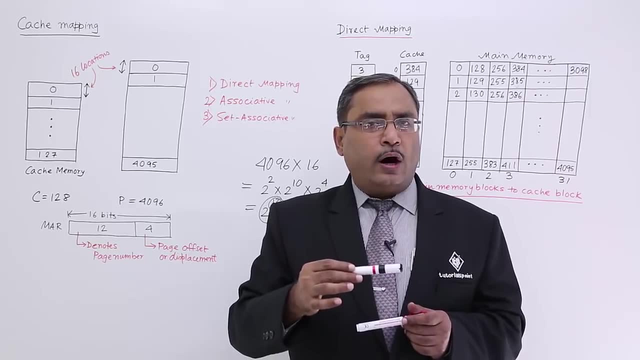 instruction which is executing now and the next instruction which is going to get executed- probabilities highest that it will be in the vicinity of the previous instruction with your current date of each entry. in this case will be in paste, but not in last pf. one is struggles the it five per day. that might be enough because the values is, because why tomorrow only one person page Раз. 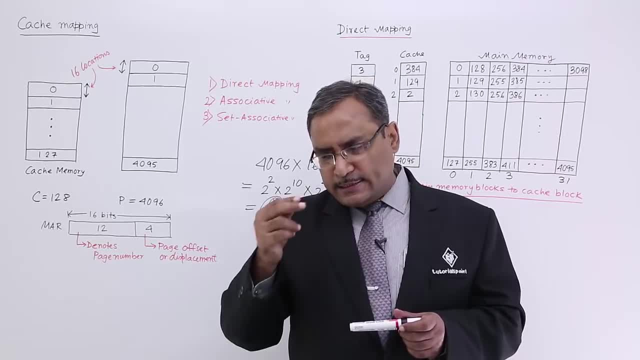 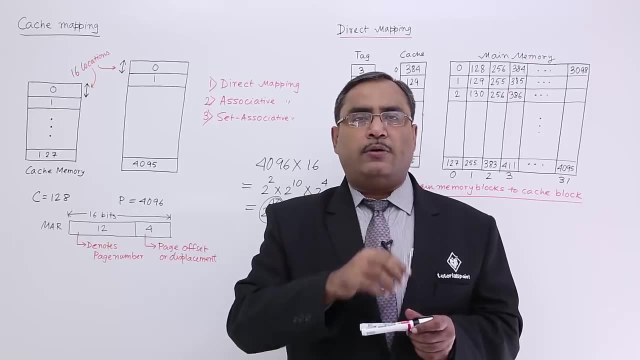 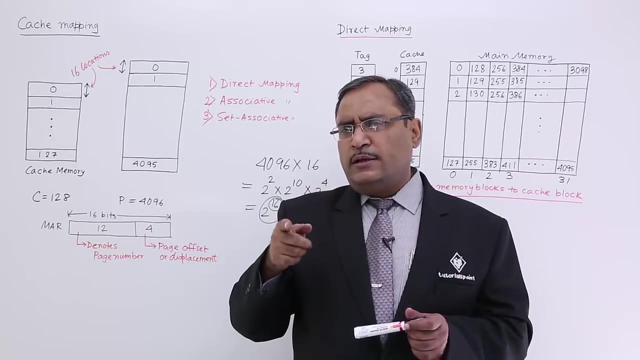 instruction which is in execution right now. that means the next instruction which is supposed to be executed will be nearby to the current instruction which is getting executed right now. this is known as locality of reference. right now i am talking about cache memory, i think. next 10 to. 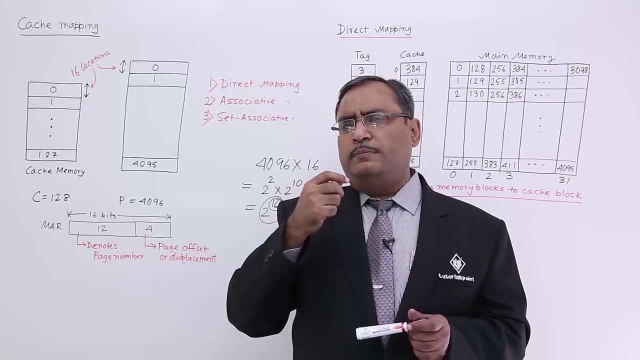 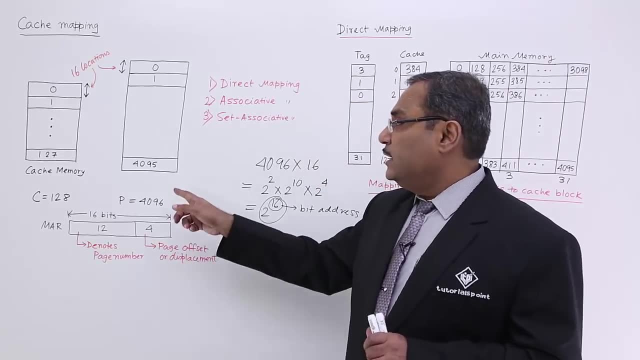 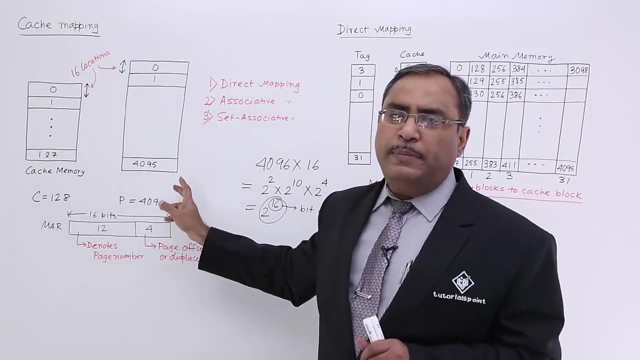 12 statements. whatever i shall, i shall make will be on cache memory also. so in my speech there is locality of reference, so that is a locality of reference. so i am i am guessing that if i load 10 locations content at a time to the cache memory from the main memory, then for the some period of 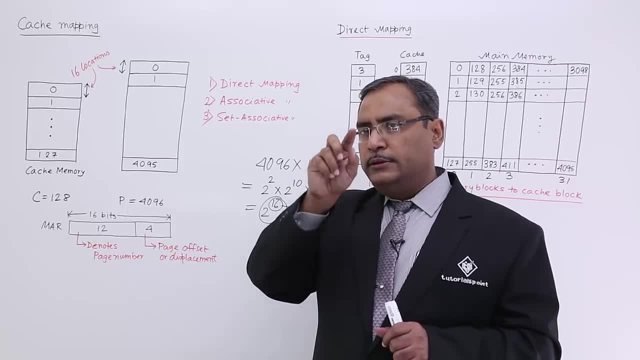 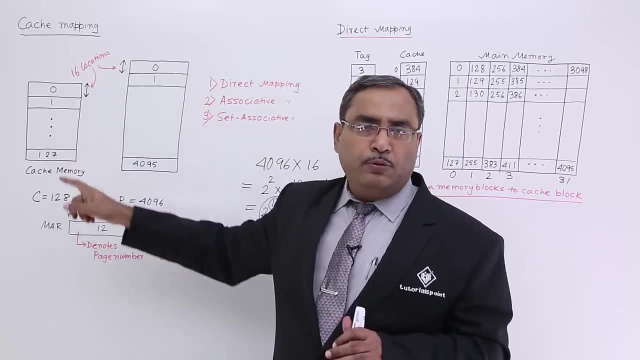 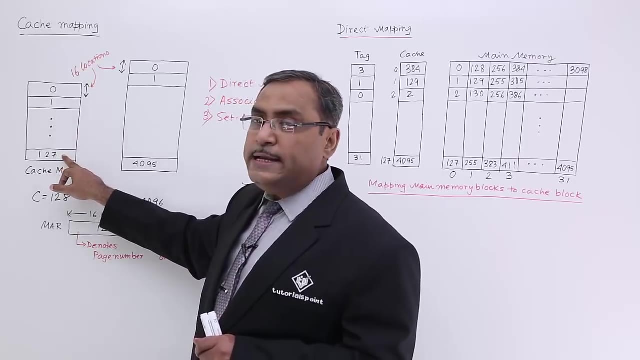 time, the program control will remain confined within that page and each and every page is of same size and in the cache memory. now let me come to the cache memory. i have divided this total cache memory into 102, sorry into 128, number of cache memory. and i have divided this total cache memory into 102, sorry into 128, number of 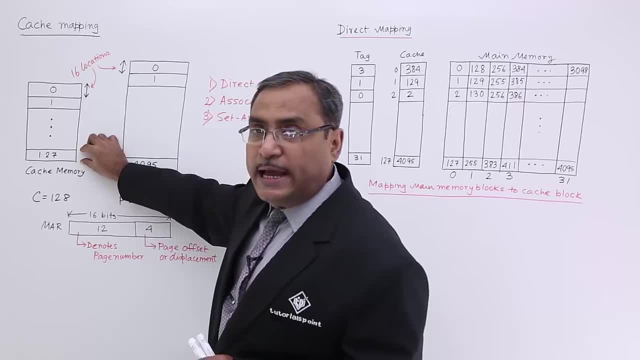 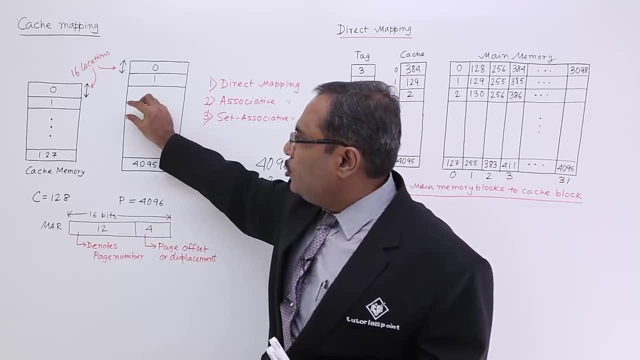 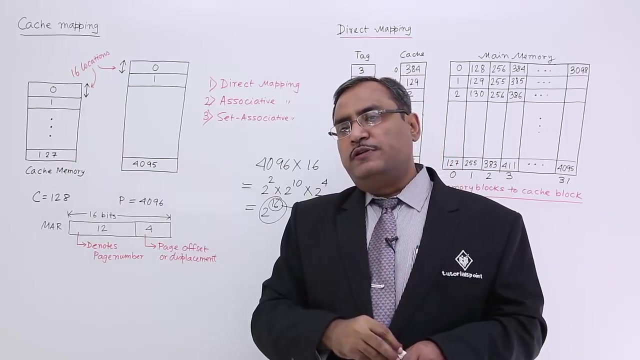 of frames where each and every frame size, each and every frame size is equal to the page size, because when one page will be going, it will be, it will fit on to a single frame. so page size is equal to frame size. that is always universally true. ok, so how many frames? 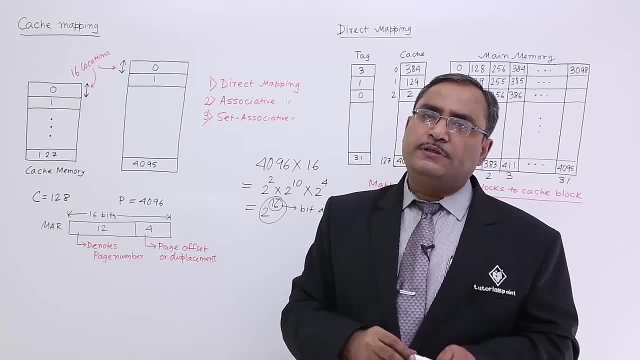 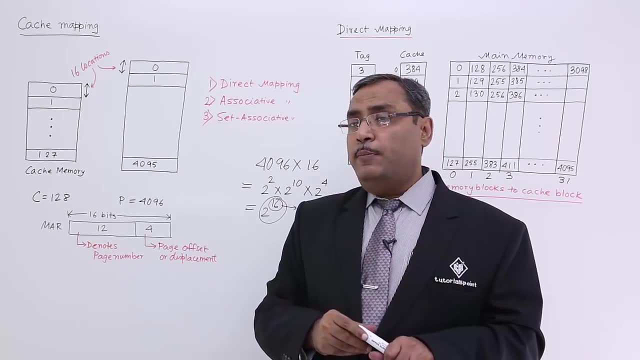 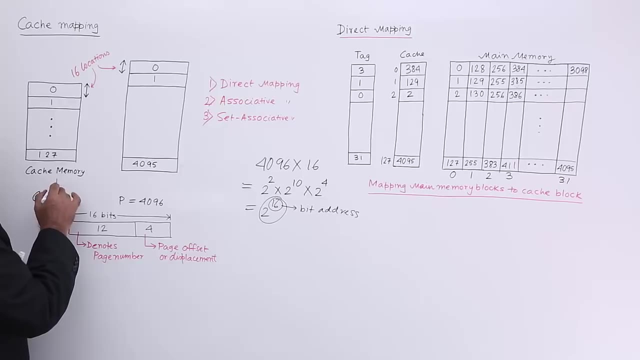 are you having in the cache memory 128 number of frames. if you start from the frame number 0, what will be the maximum frame number? obviously it is 127, so 128 number of frames are there. so if you consider, in case of cache memory, in case of cache memory, so to denote the frame, 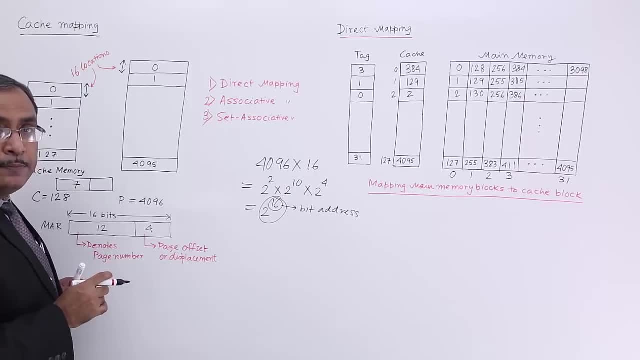 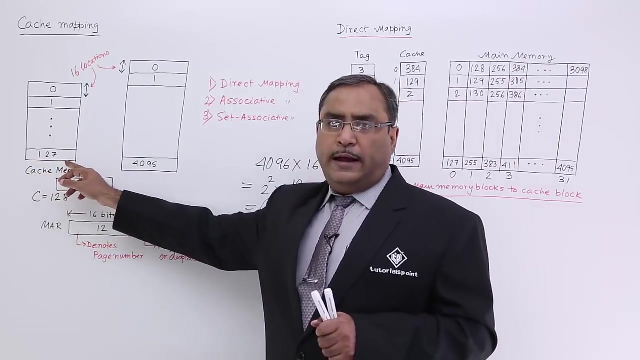 number. i require 7 bits because 7 bits can have your 128 combinations and, as i told you, that page size is equal to the frame size, so we will be having 4 bits for the page page offset or the displacement. So So cache memory at this bits will be 11 and main memory at this bits will be 16. according. 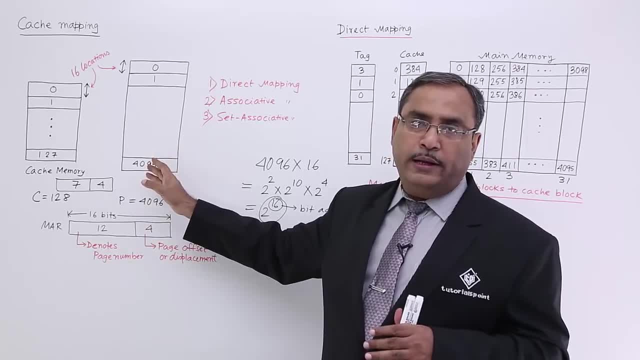 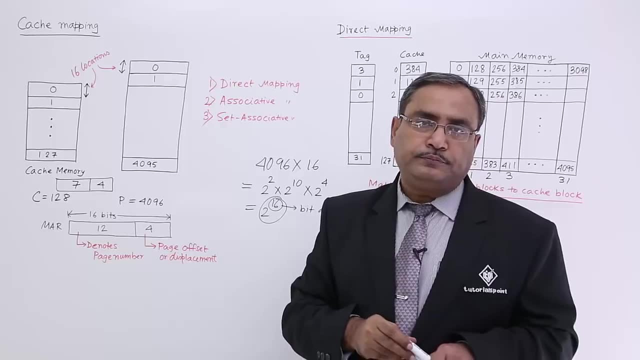 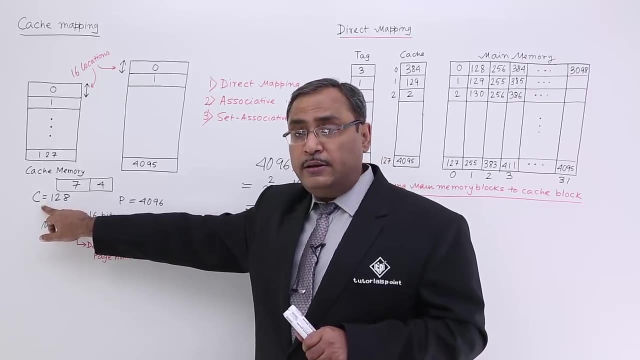 to my example. it is not hard and fast that always it will be doing like this. i am taking one example so that i can go for the mapping accordingly. so that is the way it is being done. good, next, so c is equal to 128. here c is equal to capital c. i have written so there. 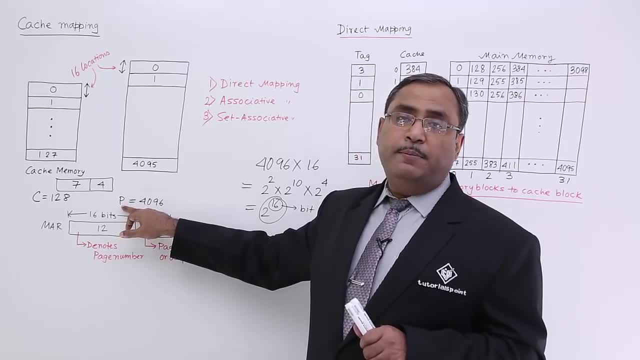 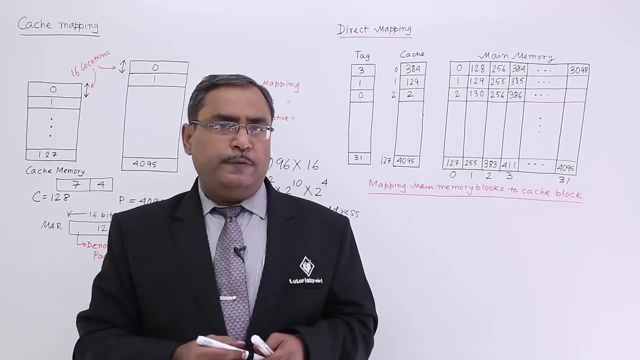 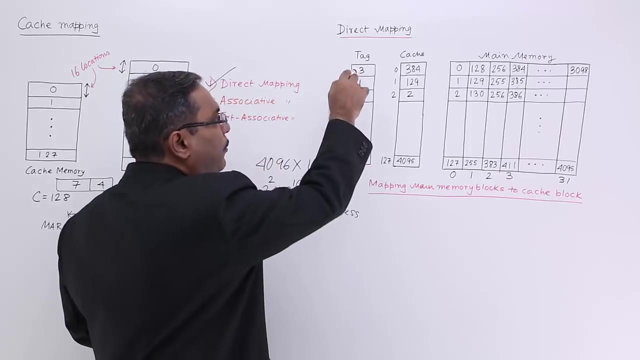 is a cache memory frame number, and here the capital p, that is the main memory page number, is 4096. now let me go for the direct mapping. so in this, in this training, we are discussing this direct mapping. ok, in case of direct mapping, what will happen? how many, how many frames? 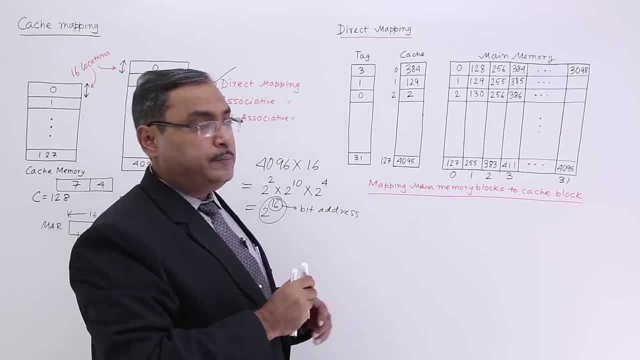 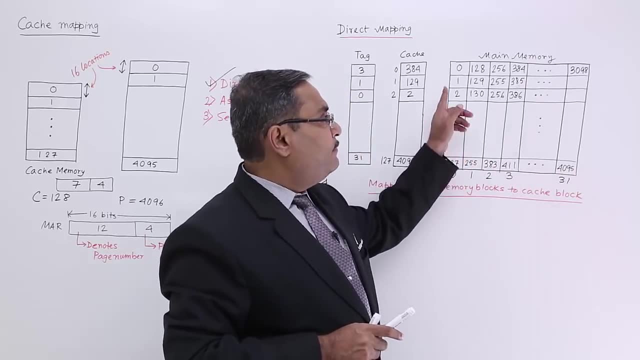 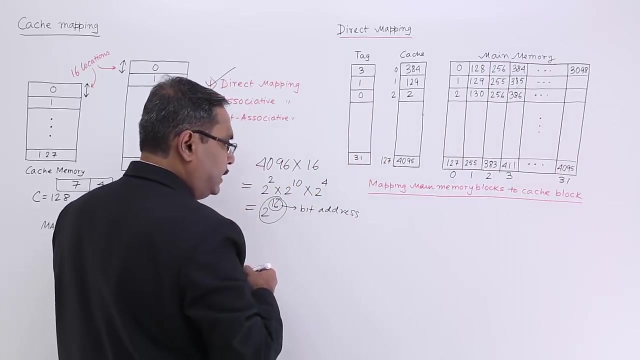 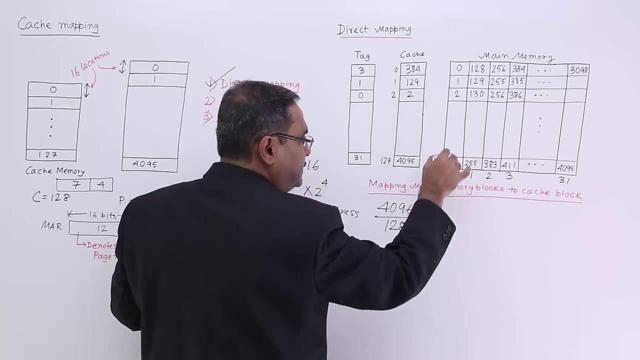 are there in the cache memory. how many frames? 128 number of frames. so i shall make 128, then 128, then 128, and so on. in this way i am dividing this main memory into 32 number of blocks. why? because you see, if 4096 is getting divided by 128, because 128 pages in a single block. 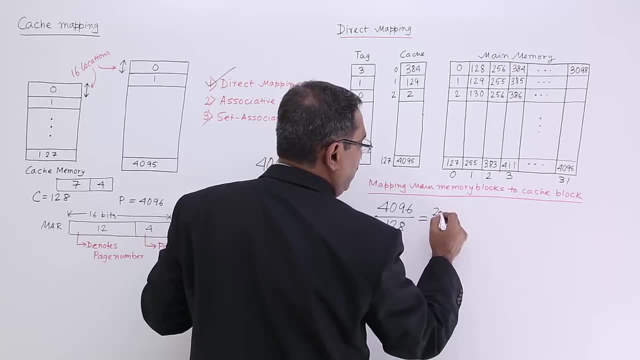 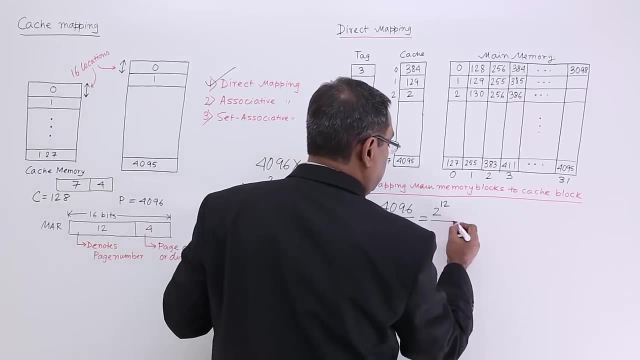 in this way, i am having 4096. what is this? it is 2 to the power of, it is 2 to the power of 12, 4096 is 2 to the power of 12, and this is nothing but 2 to the power of 7. so when 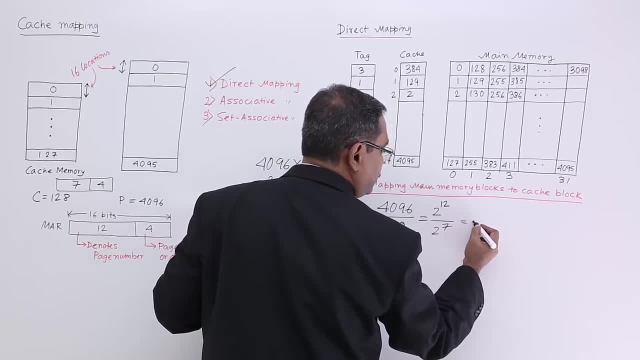 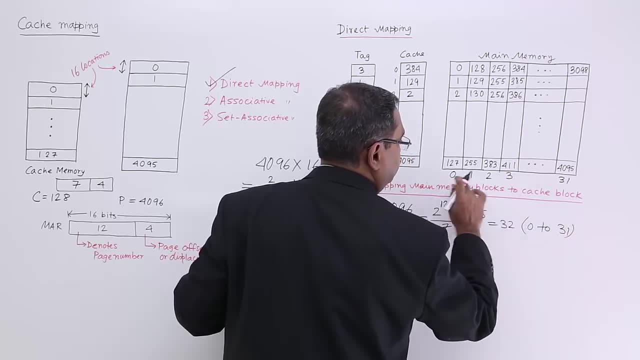 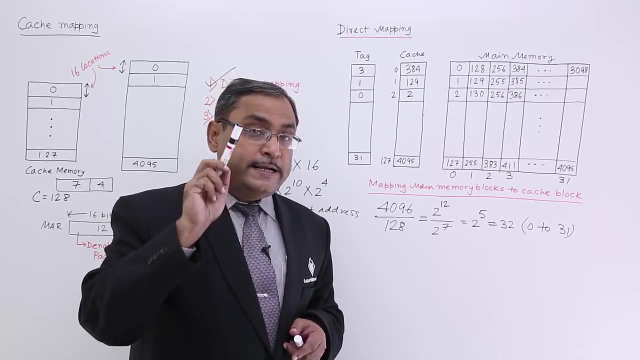 the bases are equal, then exponents will be subtracted in case of division. so 2 to the power of 5, and that is 32.. that means 0 to 31. 0 to 31. now please remember what is the name of that mapping: direct mapping. 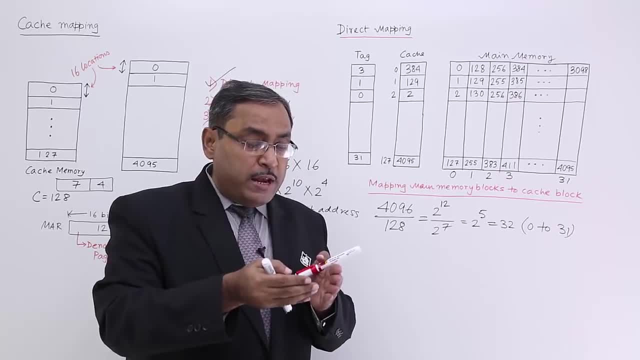 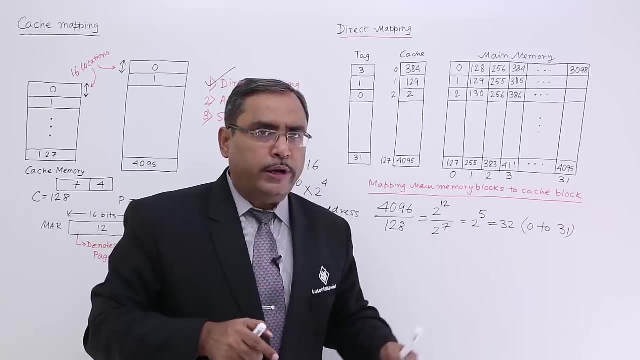 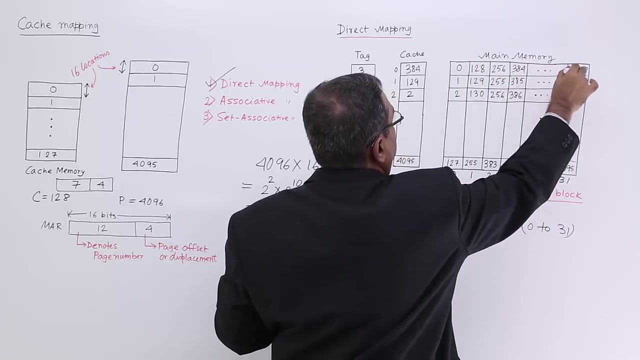 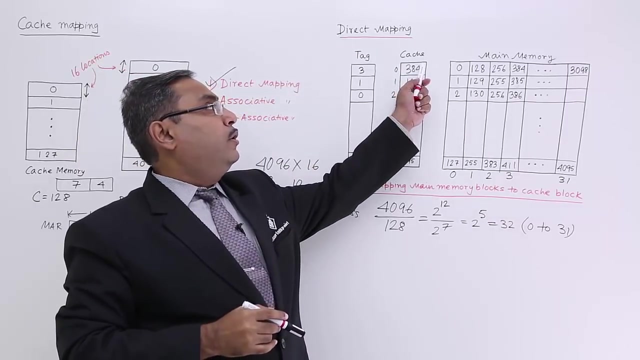 means what? from the from the main memory page number directly, i can tell you to which frame of the cache memory it is going to get loaded. so all this, all this 32 number of all, this 32 number of pages are probable to get loaded here, all of them. but how many page can be loaded on? 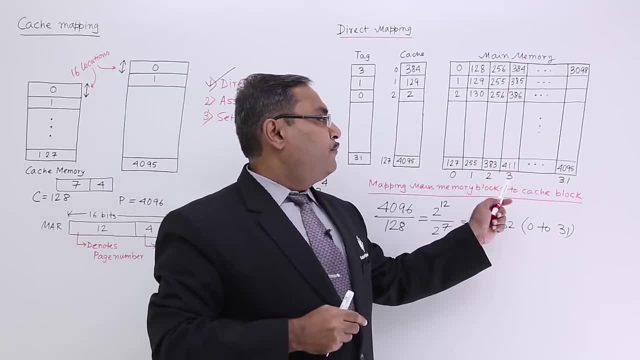 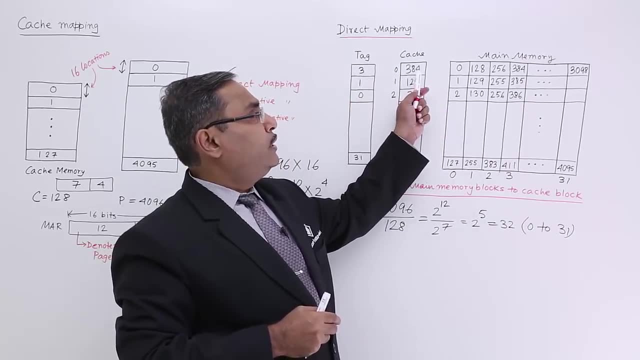 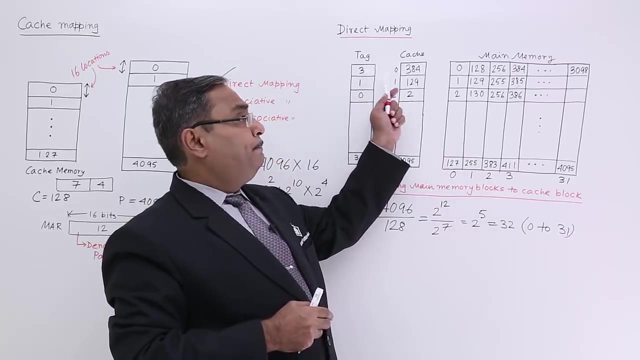 on a single frame, only one. so from which, from which block, it has come? that will be denoted by the respective tag number. so which page has got loaded here? 384 384 is having the tag number 3, so there is a tag 3 in this particular frame. which pages can get loaded? this pages? 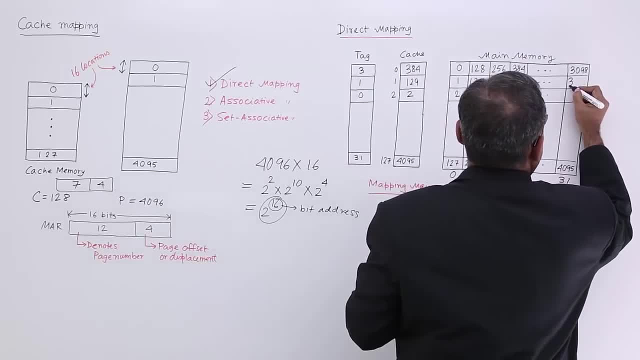 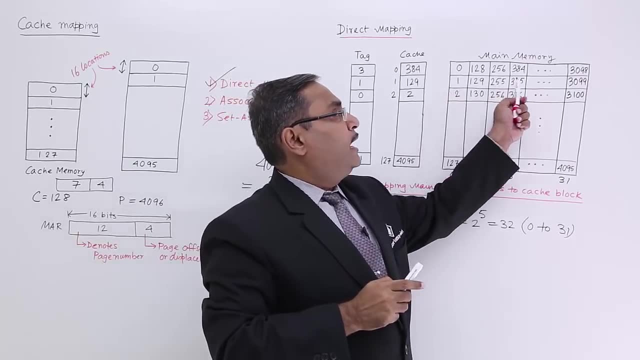 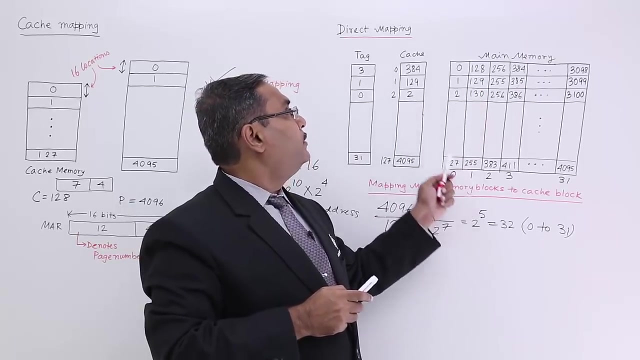 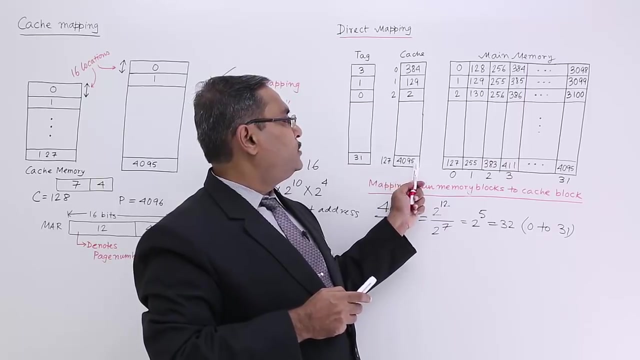 can get loaded, so it is also 3099. it is 3100. ok in this way. so now these pages are probable to get loaded here. which page has got loaded? 129. it came from which tag 1? which page has got loaded? 2? which tag 0? which page has got loaded? the last one? which tag 31? so that is the logic. 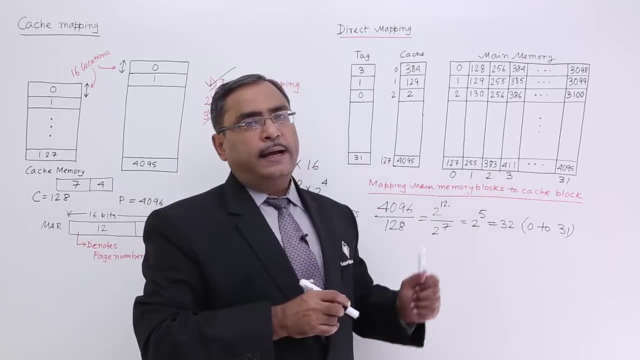 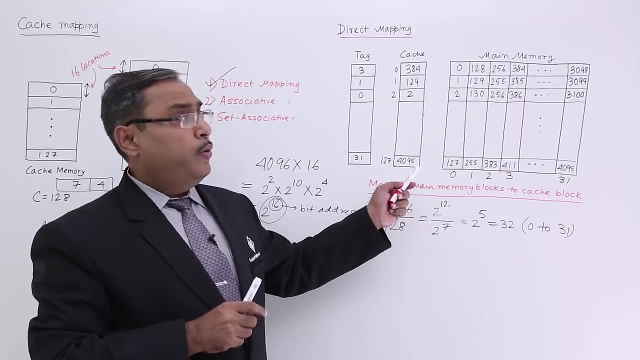 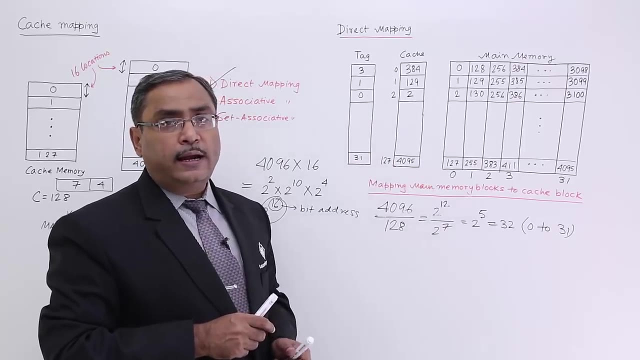 of this. that is the logic of this. so in this way i am getting the idea. ok, so this is known as direct mapping, where which page of the main memory is getting loaded on to the cache memory, that can be decided in this particular diagram. so this diagram is very attractive and very easy to understand. 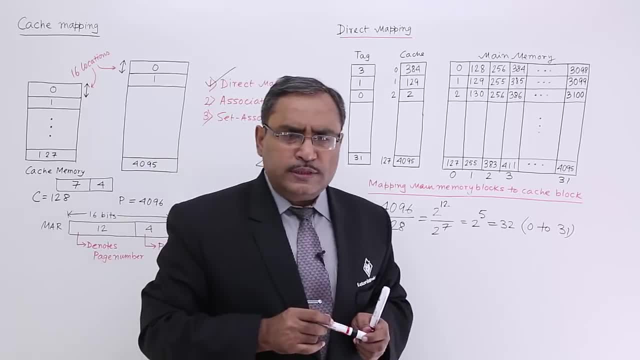 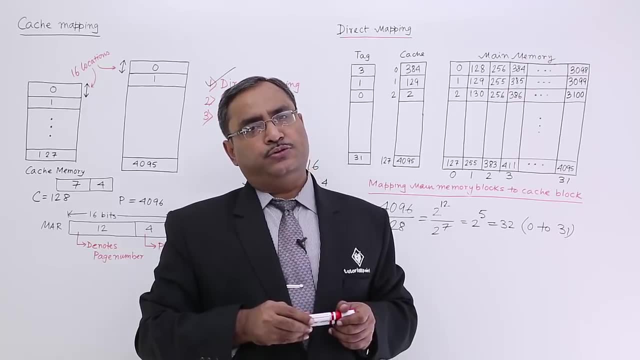 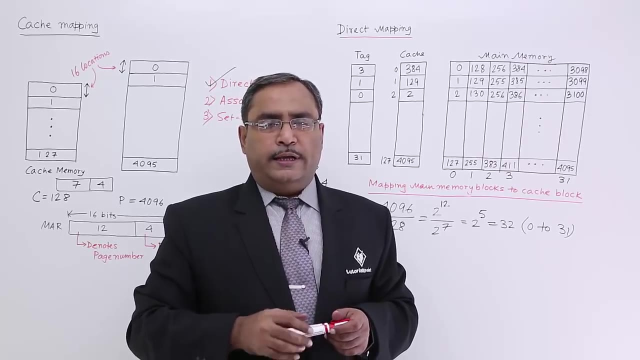 that which page is going. so now the thing is that one question might come that in case of direct mapping, which page replacement algorithm has to be used. actually, we shall go for the page replacement algorithm later, but if you know you can get my point here. you see, there is no page, no page replacement. 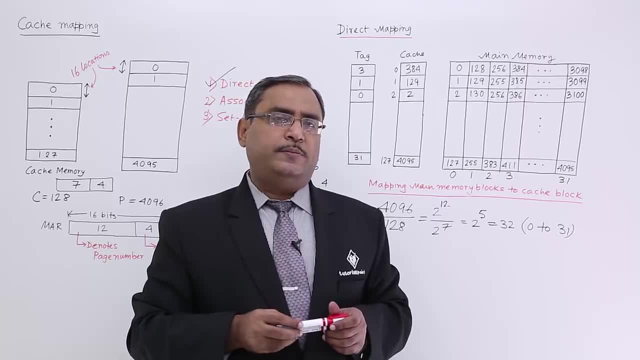 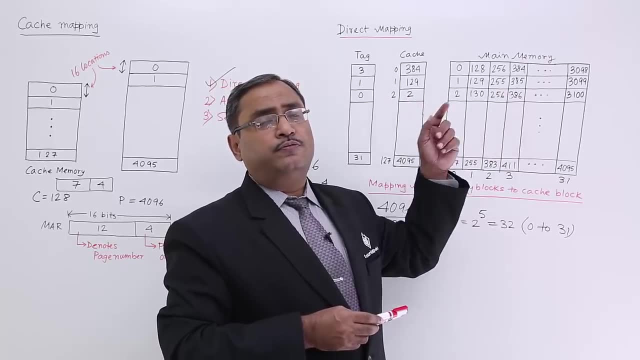 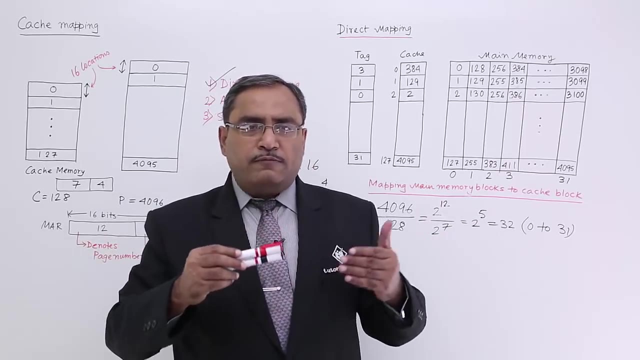 algorithm. no page replacement algorithm will be used in case of direct mapping, because from the very page number i can easily get the respective frame number, so to which page, to which frame it is getting directed. so it is quite common, so there is no need to perform any page replacement algorithm. let us suppose i am having a confirm ticket. i am having 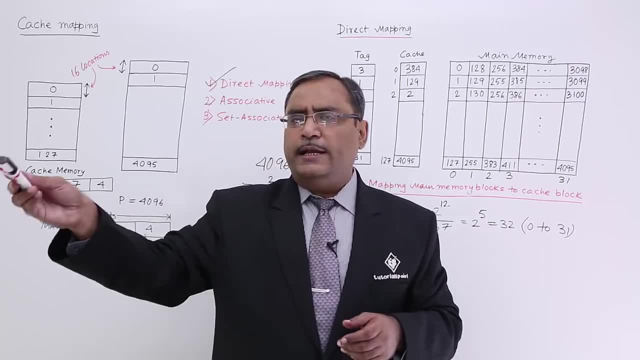 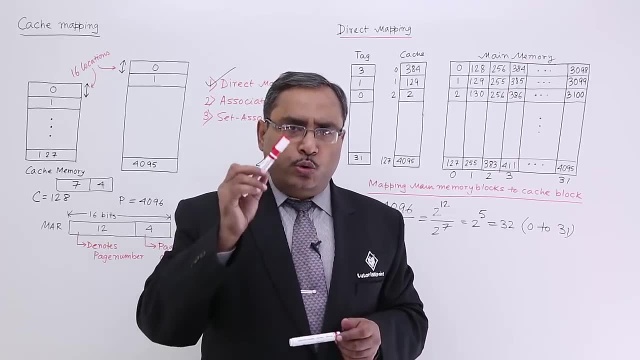 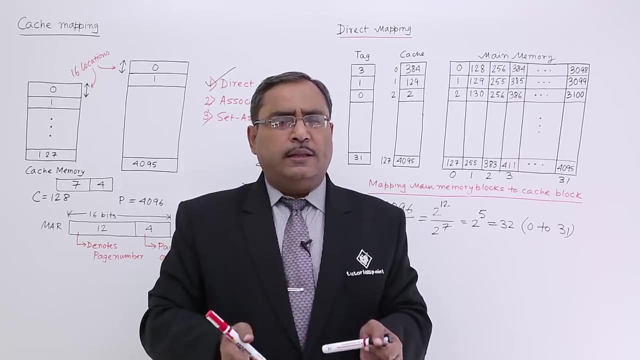 a confirm ticket on rail. ok, after entering into my compartment, i am finding that all seats are occupied. then which person? to which person should i request to make my seat vacant? which person? the person who is sitting in my seat number. so that is no replacement algorithm is required. 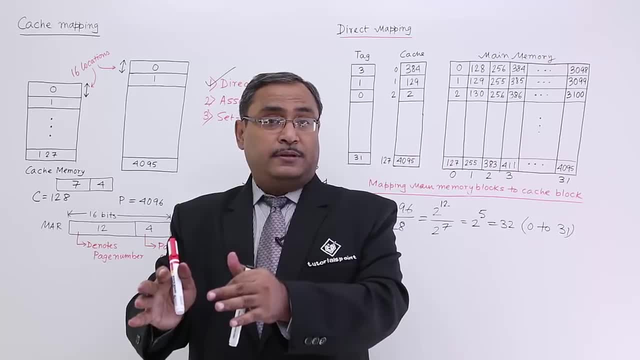 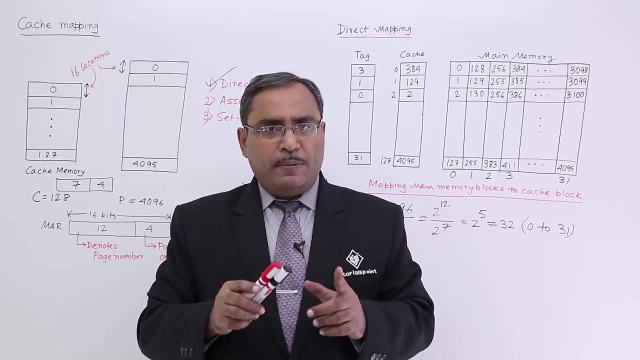 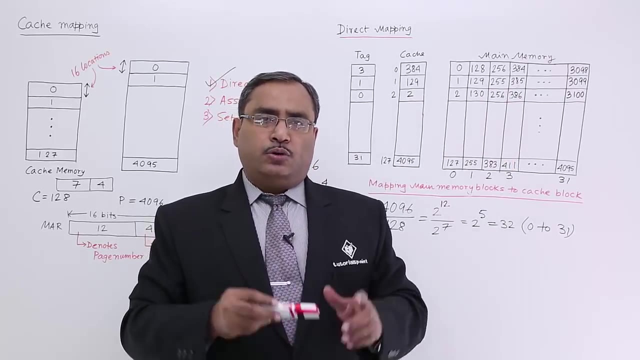 i know that i should request that person that he might, due to some mistake, might have seated in my, in my seat. so that is why, in case of direct mapping, there is no page replacement algorithm, because from the very page number i can easily get the frame number. so that is the end of this particular direct mapping. we will be